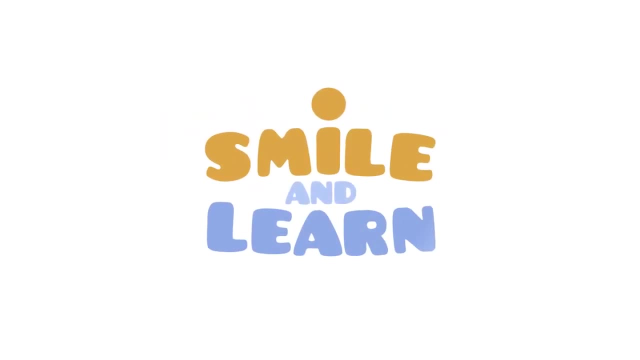 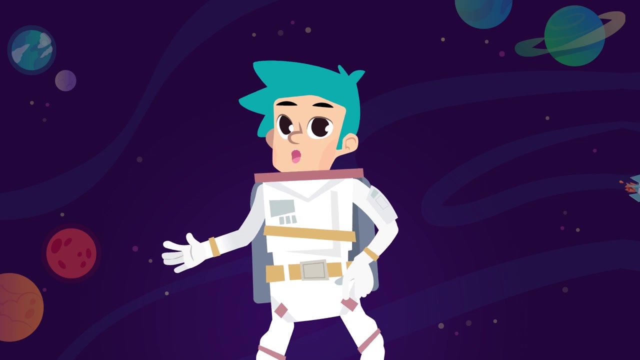 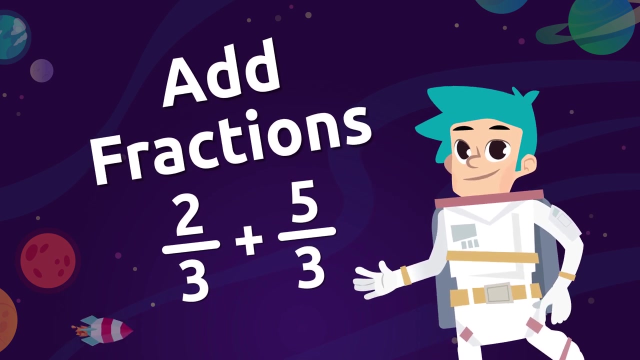 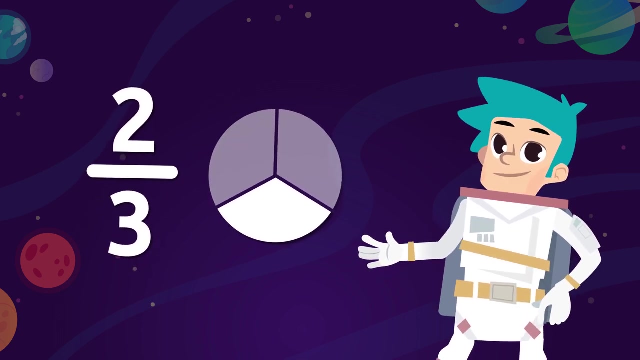 Hello again, math friends. Today I'm here so that we can learn all together how to add fractions with the same denominator. Do you remember what a fraction is? A fraction is a number which indicates the division of a whole number in equal parts. First, let's 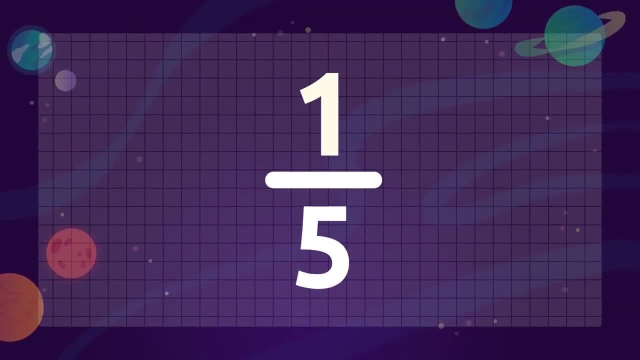 remember which are the parts of a fraction. This is the numerator and this number is the denominator. Today, we're going to take one step further. We'll learn how to add fractions. To add fractions with the same denominator, we leave the common denominator and add the. 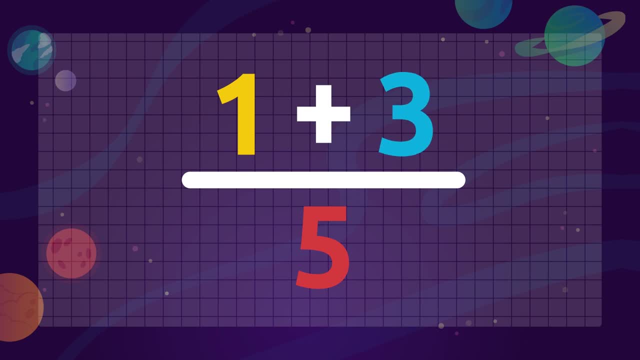 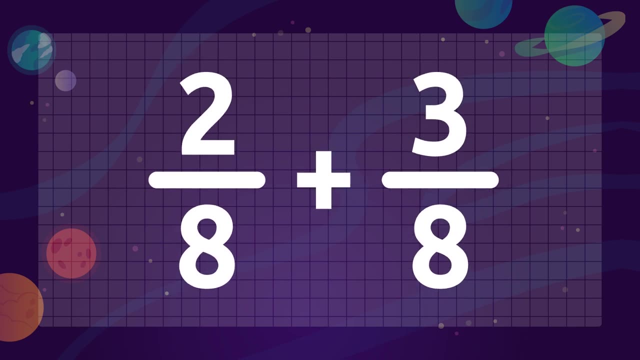 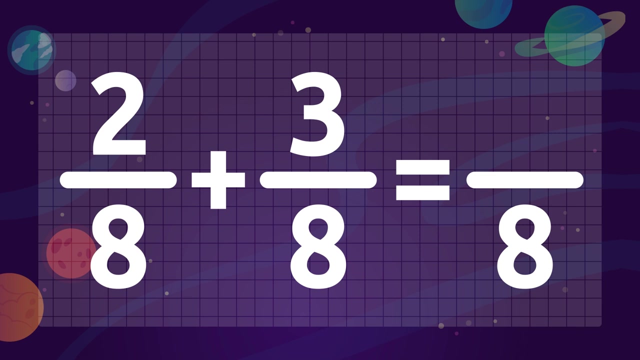 numerators. It's very simple. Let's see an example. To add 2 over 8 plus 3 over 8,, we leave the common denominator- in this case it's number 8, and we add the numerators. that is 2 plus 3, which equals 5.. This result- number 5, will be the numerator. The result is 5. 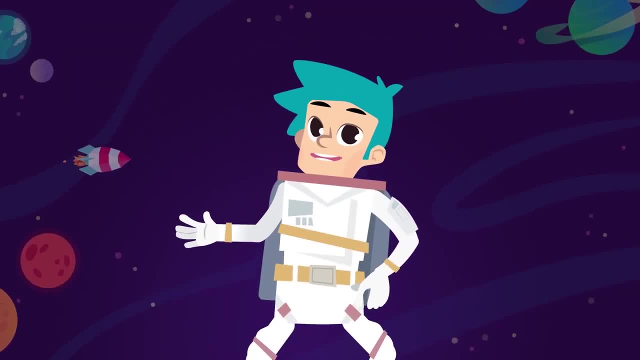 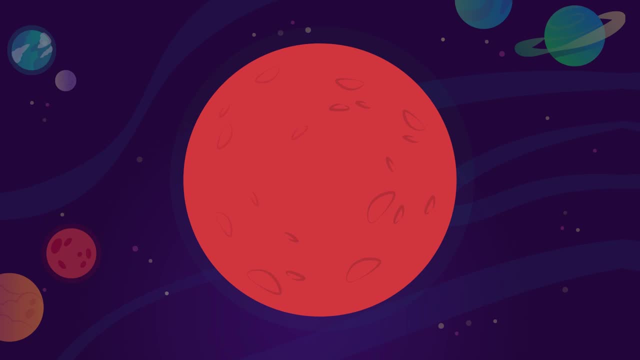 over 8.. Are you up for a challenge to practice a bit more? In the Smile and Learn universe there's a planet called Smileython. This planet is divided into eight equal parts. Two eighths of the planet are occupied by friendly aliens. 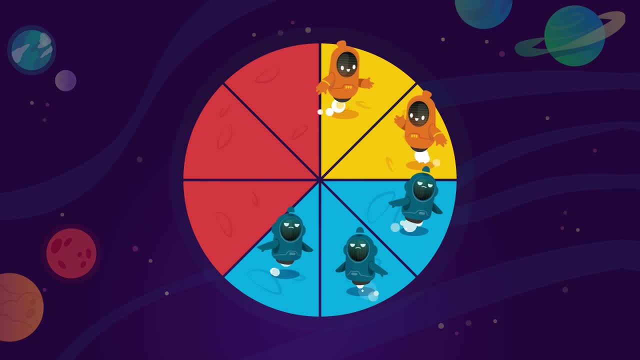 and the remaining three eighths by grumpy aliens. What fraction would represent the overall number of land occupied by all of the aliens on the planet? To find out, we'll need to add the fractions. 1 is the number of secondkę, 2 is the denominator and 2 over 8 is the agency That. automata square brake represents how much weight adds our 축. The number of times pirate is a factor too. However, that Data Sum is supposed to include the number of times in the excellent calculator and the first weak element of abenτέ. So trobance is a logical expression of 9 times cos. but 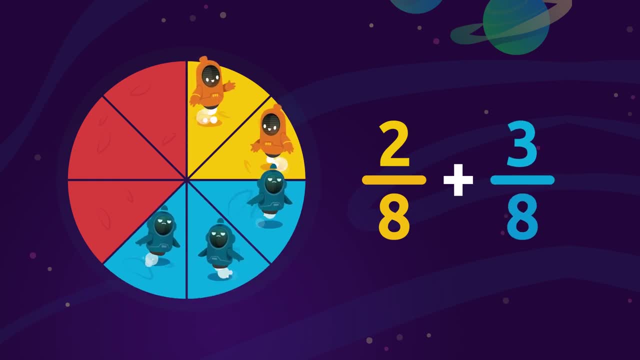 of the seventy two dayación and the number to throughput is 3 over 8, plus the number 8 times oganParkov. To get this expression right, we need to learn to complement the function of one declining selber or Plus three over eight. Do you remember how to do this math operation? 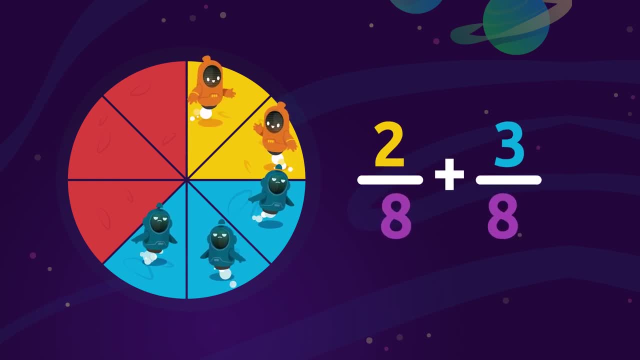 Remember that the result would have to be the same denominator. in this case It would be the number eight. and now to calculate the numerator, We'll add the numerators two and three, which equals five. The result will be that five eighths of the land are occupied by aliens.